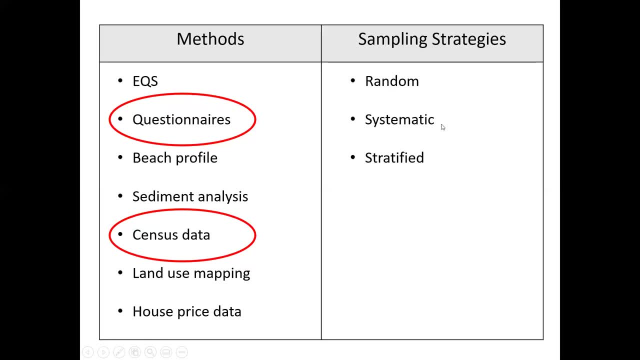 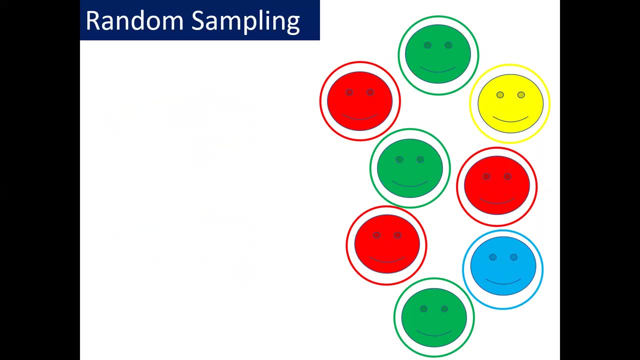 strategies. These are the only three you need to know about: Random, systematic and stratified. Okay, let's begin with random sampling. The key thing about random sampling is that everybody has an equal opportunity of being picked. Okay, so, everybody has an equal opportunity of being picked. Now, with random sampling, you don't simply 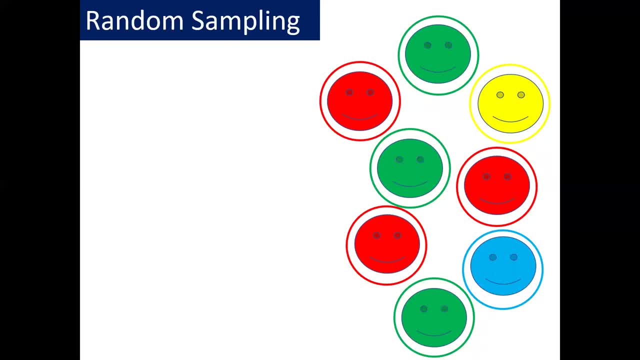 choose somebody at random. So, for example, my favourite colour is red. therefore, I'm more likely to pick the red person on here. What we use is a random number generator and this will give you a number. So it may give you the number four, for example. So you would count one, two. 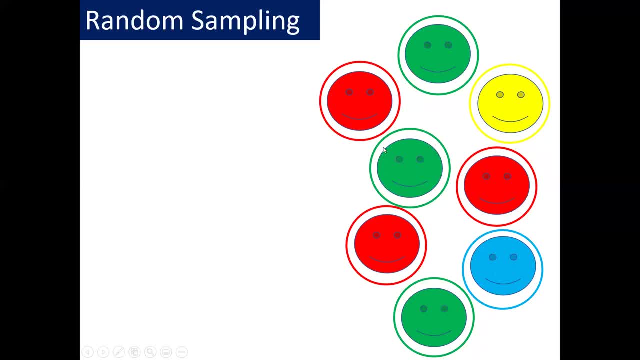 three, four and that would be the piece of data that you pick. Okay, so here we've got eight pieces of data. We've got three red faces, three green faces, one yellow face and one blue face. Okay, the advantages of random sampling: it reduces bias. So, as I said to you earlier, you may pick the. 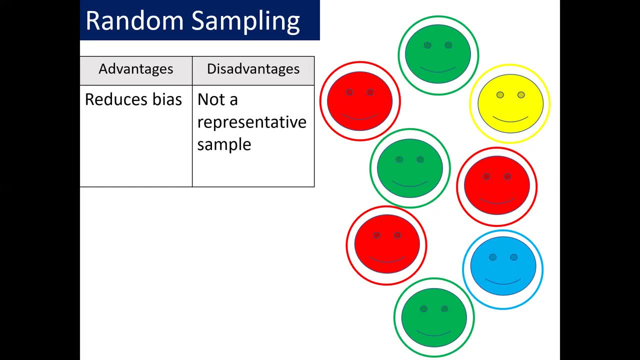 person nearest to you or the person with the friendliest face, or whatever. This random sampling reduces bias and stops that from happening. However, a key disadvantage is it's not a representative sample. So, for example, you may do a random number generator and it may give you the number. 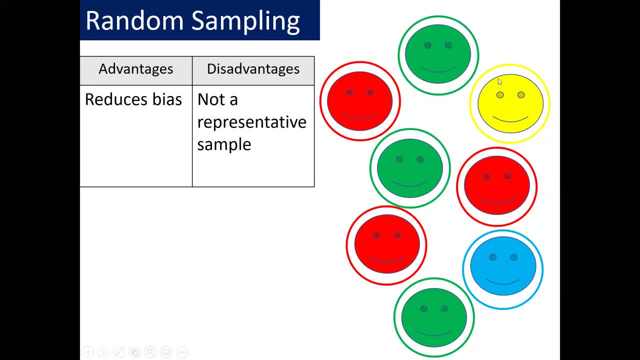 three. If we go one, two, three, we may end up speaking to the yellow person. However, there is only one yellow person on here. Most people are green or red. Therefore, it would not be a representative sample And we use random sampling or our sediment analysis in the coastal field work. That's the only time we use. 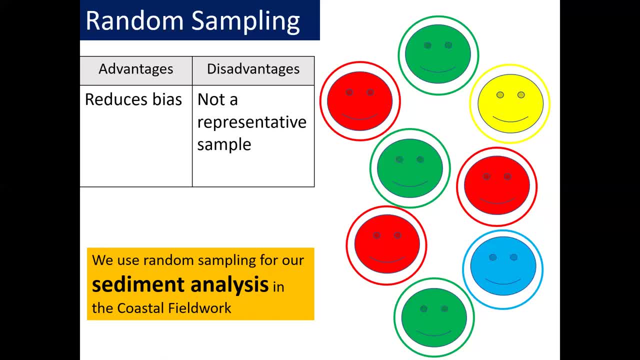 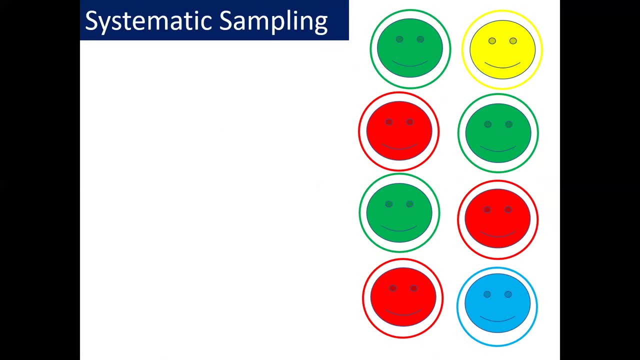 it. So we're not going to use random sampling or random sampling in our work. Okay, systematic sampling Now. systematic sampling is fairly easy to do, So we use it quite a lot in year 10 and year 11.. Again, we have eight different pieces of data here, So eight different faces on 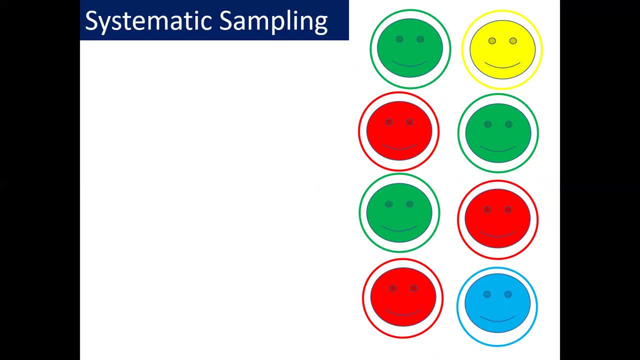 here Now. the key thing about systematic sampling is that we use intervals, So we collect the data at intervals. It could be based on time, So, for example, you may choose to pick your data every two minutes. It could be based on distance, So, for example, you may decide to stop every 200 meters along a road. 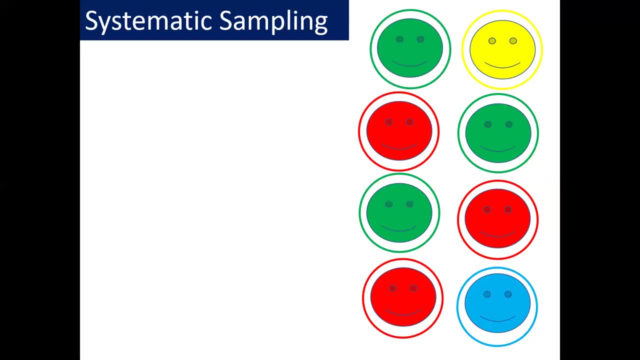 and collect your data there. So there's lots of different ways we can use systematic sampling. As an example, here we're going to pick every second person, So you can see the yellow person's picked, the green person, the red person and the blue person. So we've ignored these people here. 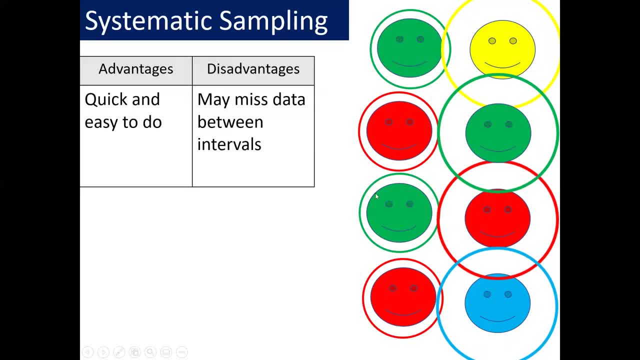 here and we picked every second person. Now, the good thing about systematic sampling is it's very quick and easy to do, So you can turn up at a location and you can do your systematic sample very quickly and set it up very easily. However, a key disadvantage is that you may miss data between the intervals. So 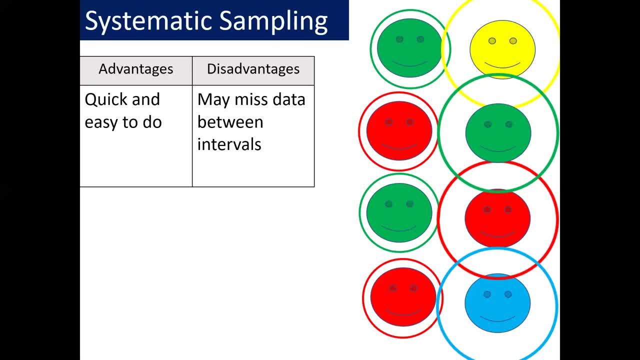 for example, if you are collecting data along a road and you're stopping every 200 meters, there may be some really important data at 100 meters that may be missed. Similarly, here, the red person may have some really important data that we want, but that person gets missed because we're only picking every second person. 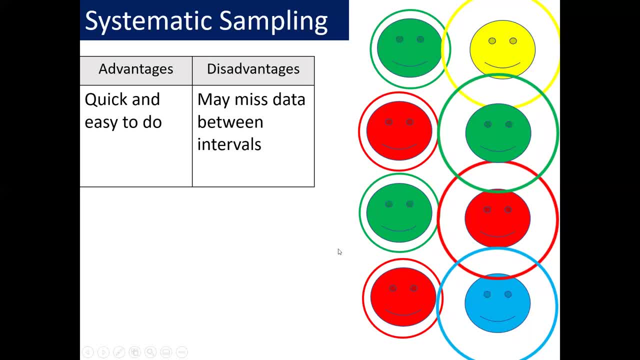 Remember, systematic sampling is done at intervals. Now, because it's quick and easy to do, we use systematic sampling for our beach profile in the coastal field work And our land use mapping and EQS in the urban field work. Okay, the last type of sampling, and probably the most difficult, is what we 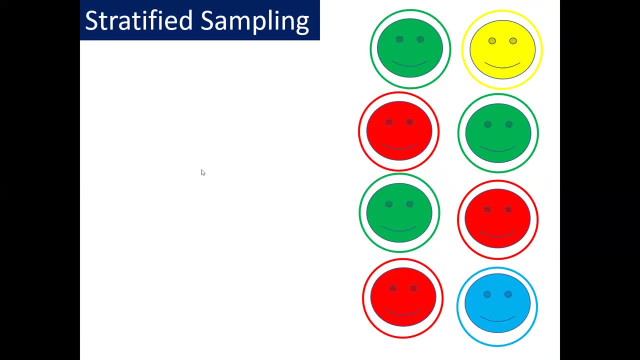 call stratified sampling. Now, stratifying something means putting it into layers. That gives you a bit of an idea of how this sampling works. Again, we've got eight people here. Now this time we need to think about who we've actually got in. 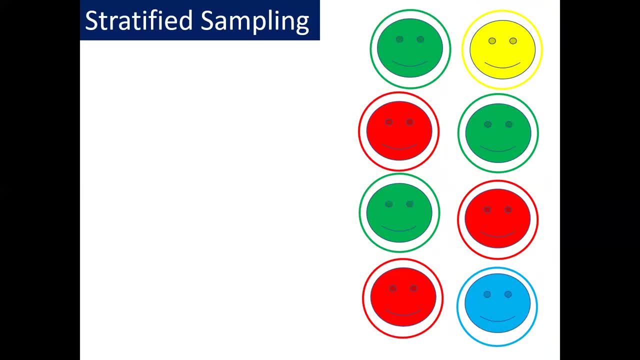 our data. So we've got three green people, we've got three red people, only one yellow person and only one blue person. Therefore, to make this sample stratified, we need to speak some more green people and more red people. So what we could do is we could speak to the yellow person. 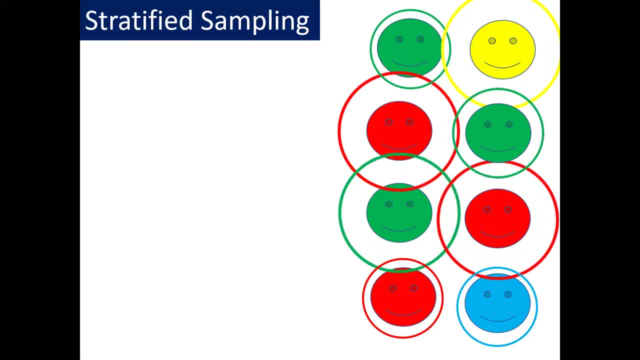 we could speak to two of the red people, two of the green people and the blue person. Therefore, our data is going to include more information from the red and green people, and that's because there are more of them in the population. So the advantage of this is.